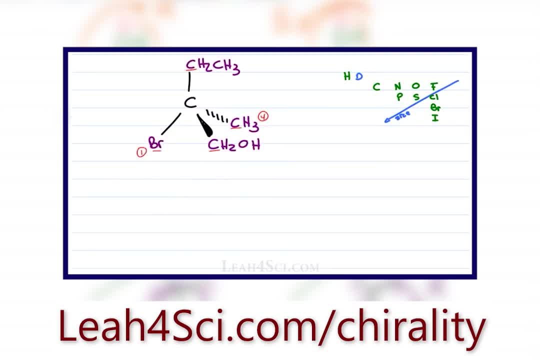 In previous videos at leah4scicom- slash chirality- linked below, we looked at how to find chiral centers and designate R and S, no matter how it's presented. In this Leah4Sci video, we'll look at what happens when a molecule has more than one chiral center. 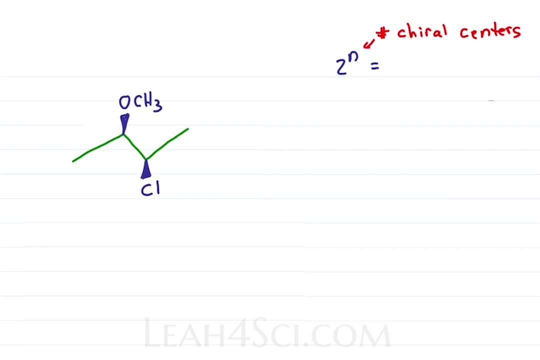 If a molecule has more than one chiral center, we use 2 to the n to find the maximum number of potential stereoisomers. where, in this molecule, OCH3 and chlorine both sit on a chiral carbon, And if n is equal to the number of chiral centers, we have a maximum of four potential stereoisomers. 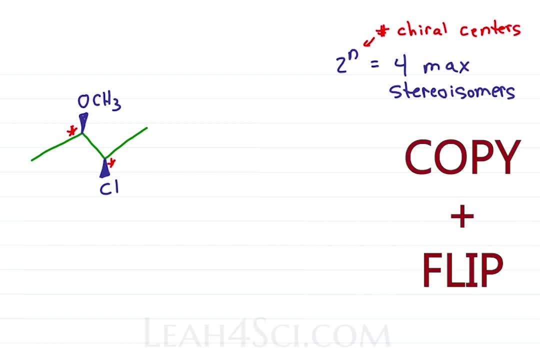 Let's find them all using a simple copy and flip method. I start with the skeletons and then I copy the substituent and flip the chirality. On the right, the starting molecule has two wedges, so we put both substituents on dashes. For this next one, I'll keep the first substituent the same and flip the other. 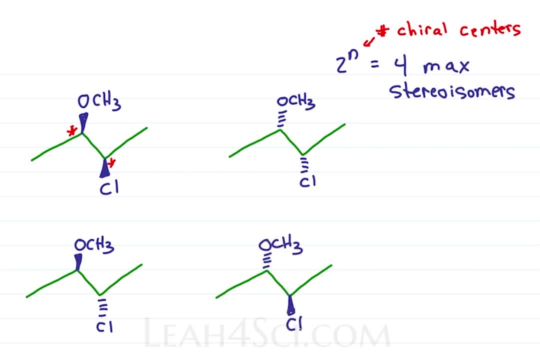 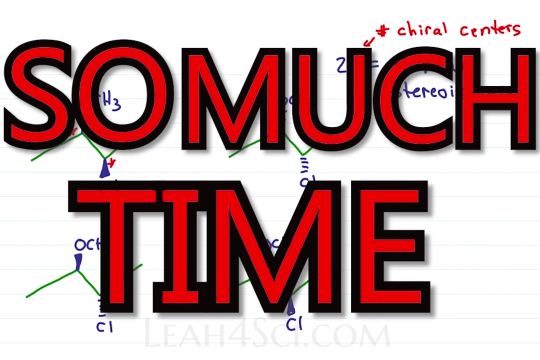 Next I'll find its mirror. by flipping both. Wedge becomes dash and dash becomes wedge. Now that we have the structures, let's find the relationship between them. The standard method of finding R and S for every single chiral center absolutely works, but takes so much time. 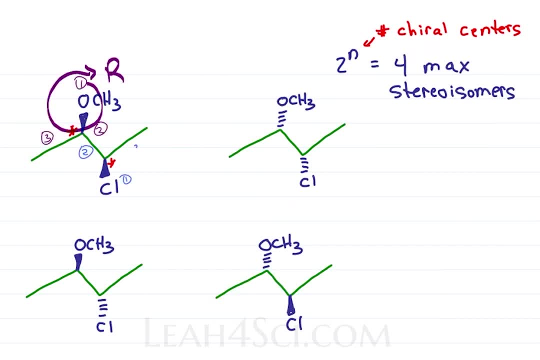 Instead, we'll solve for 1 set and then find the rest using the swap method that I teach in the videos linked below. If 1 swap gives me the enantiomer, having OCH3 on a wedge- for R means OCH3 on a wedge- If 1 swap gives me the enantiomer having OCH3 on a wedge for R means OCH3 on a wedge. If 1 swap gives me the enantiomer having OCH3 on a wedge for R, means OCH3 on a wedge. 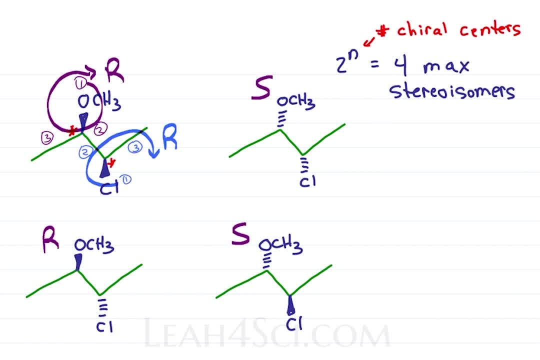 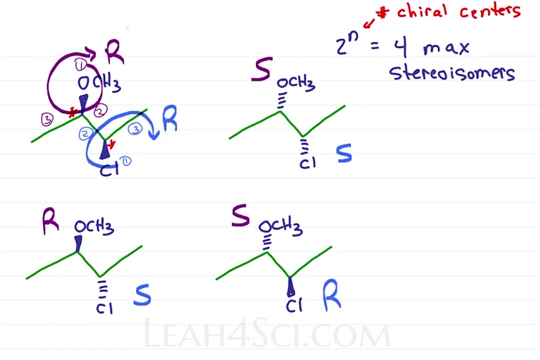 CH3 on dashes for S And wedge, of course, is still R. Same thing for chlorine: Having chlorine on a wedge gives me R, which means chlorines on dashes give me S. Not confident with the trick, Pause the video. prove the R's and S's. As for the relationships if R to S is a mirror image, 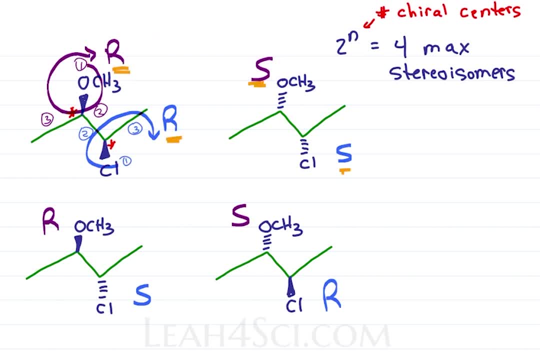 or enantiomer. when the entire molecule is mirrored, the molecules are enantiomers to each other. What if it's only partially mirrored, where I have RR on one chiral center and RS on the other? In this case, the molecule is of two minds or di-stereo minds, giving us a diastereomer. 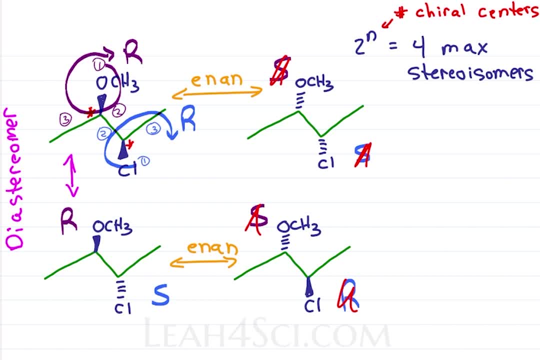 Even without the RNS designation, the quickest way to identify a diastereomer is to see that one substituent on the molecule is exactly the same and the other is opposite. This gives me another set of diastereomers, And let's not forget the corners. We have one that is different and one that is the same for another. 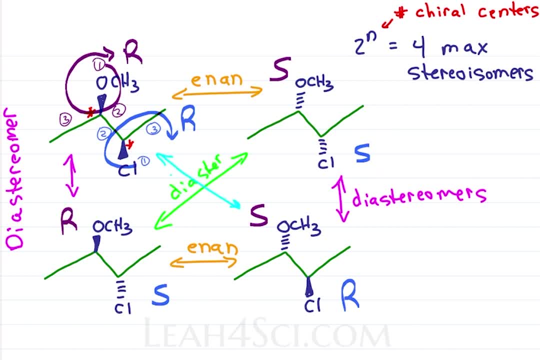 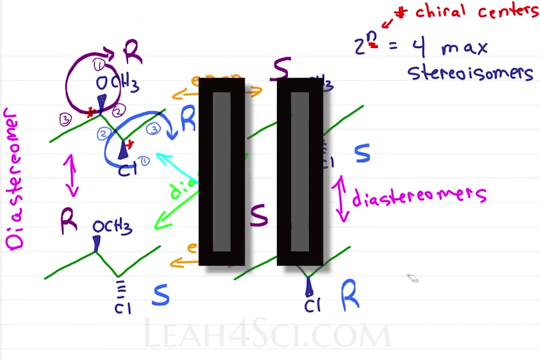 set of diastereomers And the same thing here. This became so messy, so let's summarize: If you have two chiral centers for a maximum of four potential stereoisomers, every molecule will tend to have one enantiomer and two diastereomers. Pause this video if you need a minute for it to. 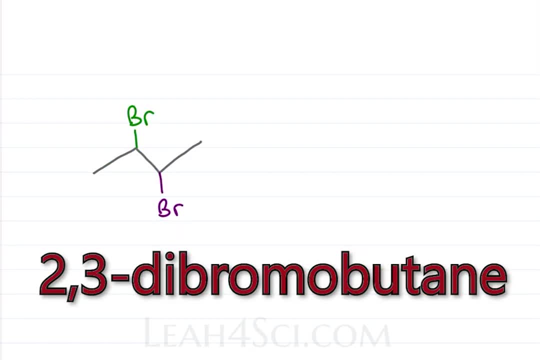 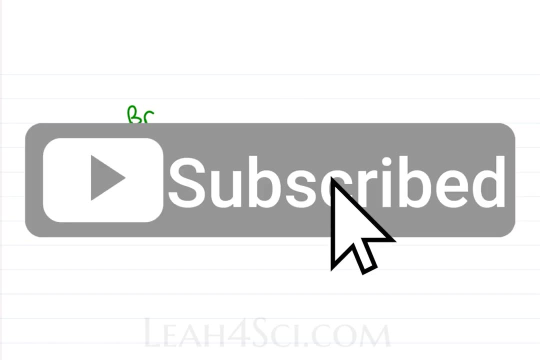 sink in and let's continue. Now let's try it with 2, 3 chromobutane. But before we dig in, make sure to give this video a thumbs up. subscribe to my channel and hit that bell icon so you don't miss out on any new videos. And let's count. 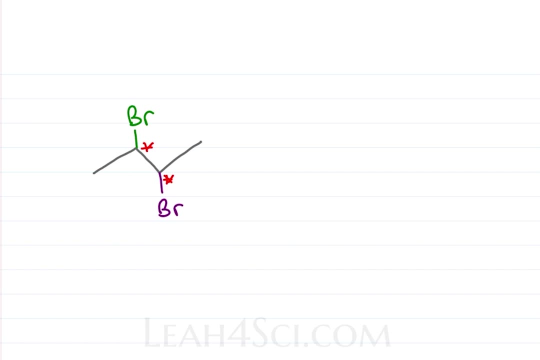 I see two chiral centers. Does that mean I have four stereoisomers, And will each molecule have one enantiomer and two diastereomers? We start with 4 skeletons and draw one chiral molecule. I'm choosing to put both bromines forward and then we'll copy and flip both chromobutanes. 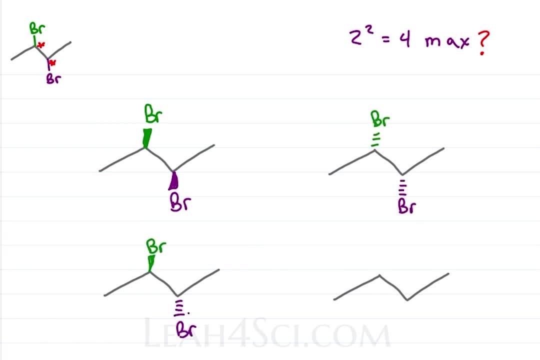 And then we'll copy and flip both bromines forward, and then we'll copy and flip both chromobutanes bromines on dashes- Keep one and flip the other, And of course it's enantiomer Next. we could 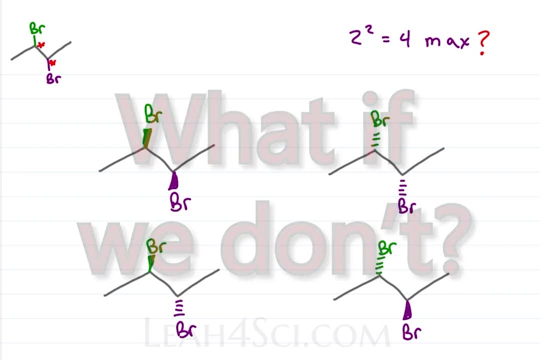 find RNS for each one. But what if we don't? What if, instead, we just look at it the way we did before? These two molecules are mirrors at every chiral center, making them enantiomers. These two appear to be mirrors as well. Are they enantiomers? Actually, no, These two are not enantiomers. 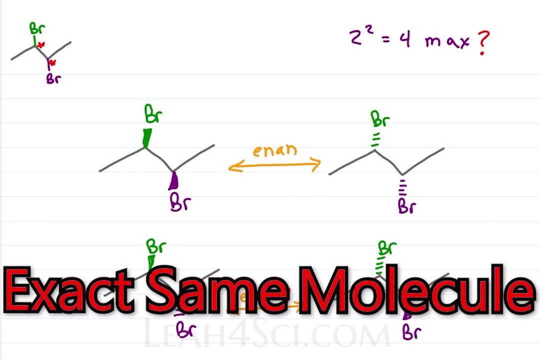 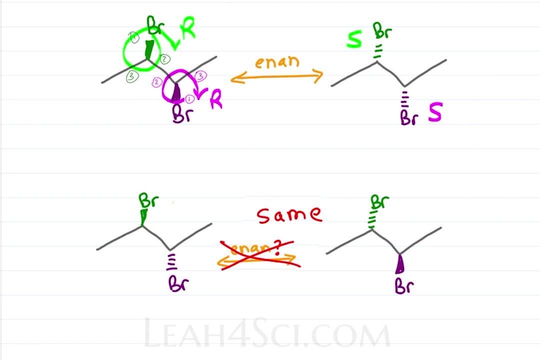 It's the exact same molecule. The green bromine is R, The purple is also R. That makes their enantiomers S and S, And on the bottom we have the green R, green S, purple S, purple R- Once again. 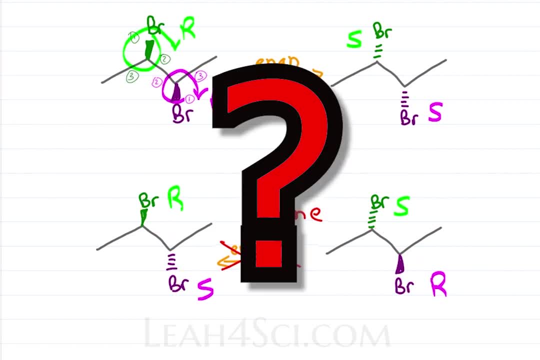 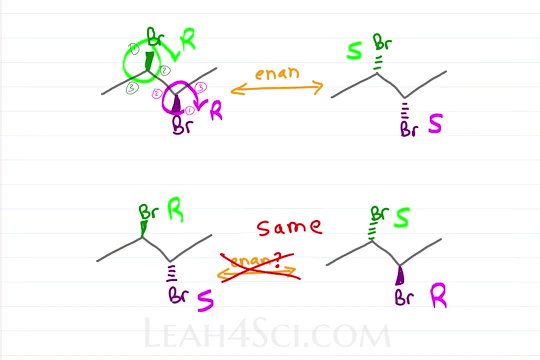 if we have R and S, then S and R, how are they not enantiomers? The difference between this and our last example is that both chiral centers have the same exact substituents. We have bromine, a methyl group, and- don't forget that- invisible hydrogen. Here I have a molecule. 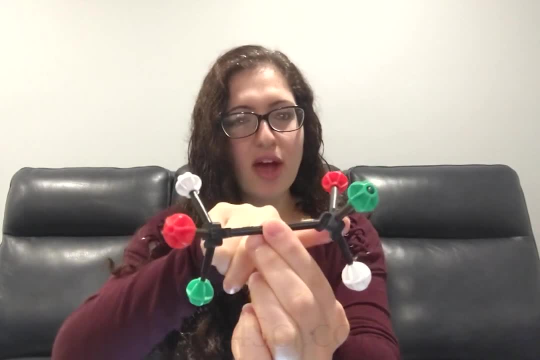 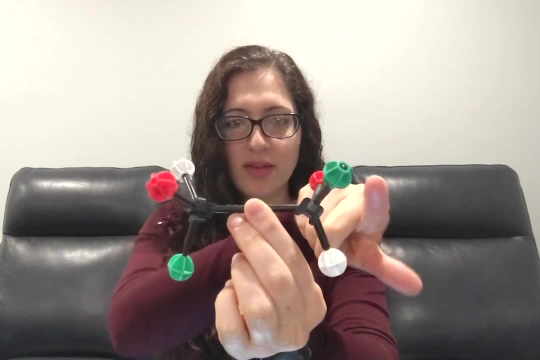 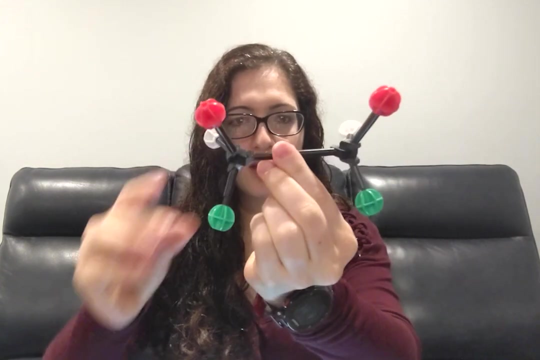 with two chiral centers, You'll notice that they each have the same four unique substituents: white, red, green and the other side, White red, green and the other side. If I rotate it, notice that internal plane of symmetry where this half is reflected and this half. 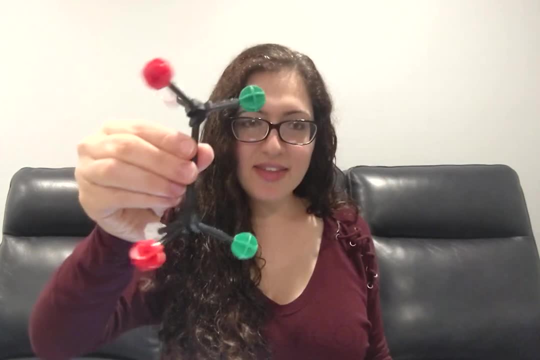 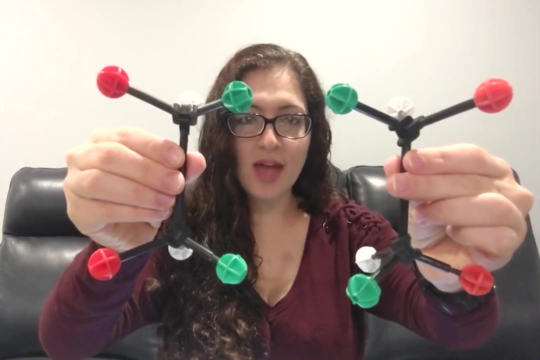 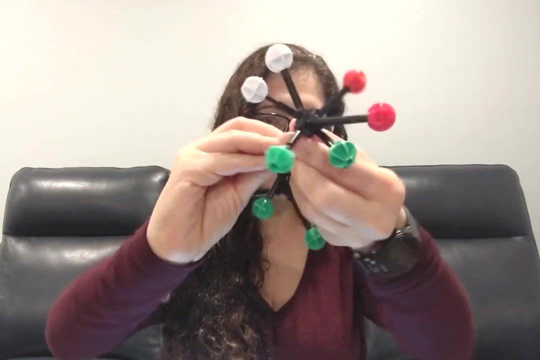 down the middle. It's exactly the same. If I take this molecule and build its mirror image, notice the plane of symmetry going down the middle. These are not enantiomers, because look at what happens when I rotate it. They are perfectly lined up. They are the same exact. 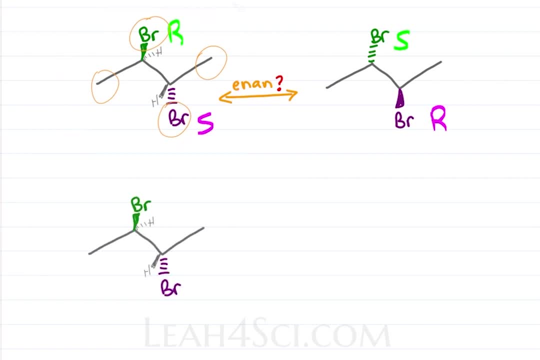 thing. Let's draw it out with this molecule And we won't look at the invisible hydrogen. We'll do a 180 degree rotation. We'll do a 180 degree rotation around the central bond between the two chiral centers. We'll tilt the. 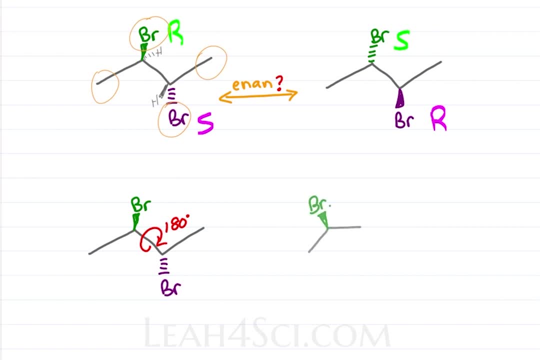 results slightly and redraw the molecule as follows. The left half doesn't change, with bromine coming out of the page. This is where I had a rotation and that gives me for the right side of the molecule where I have the purple bromine, a methyl group that is down in the plane of the page. 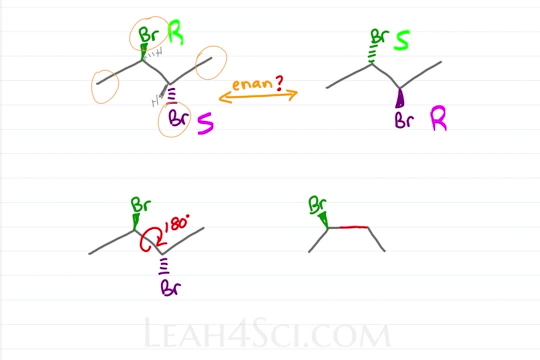 because 180 degrees from up in the plane of the page gives me down in the plane of the page. Bromine is down and into the page rotated 180, we get up and out of the page. Down becomes up, dash becomes wedge, And look at that. 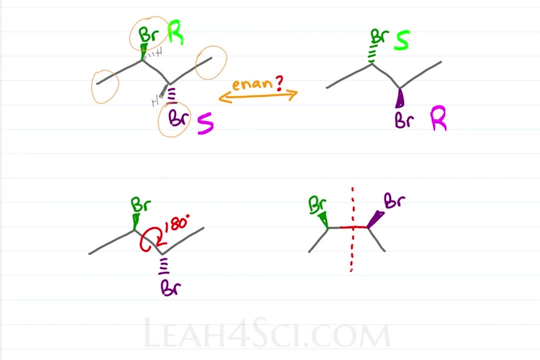 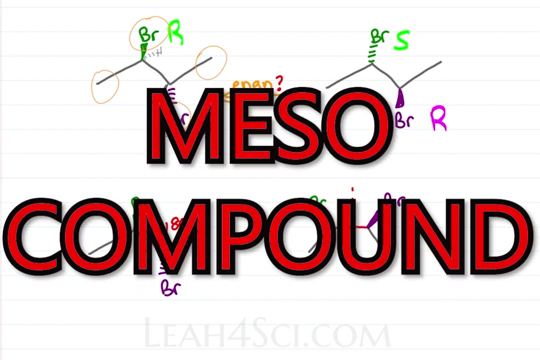 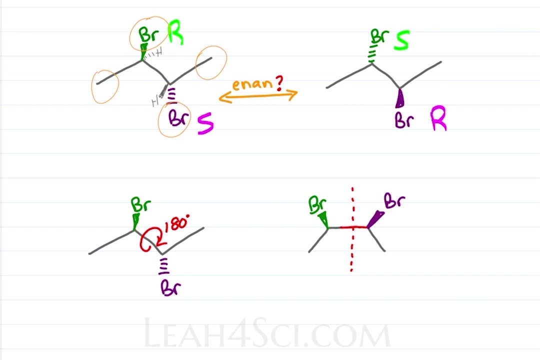 I have an internal plane of symmetry in the molecule. I have an enantiomer within the molecule itself where one half reflects on the other. This is called a meso compound And while we do have two chiral carbons, the molecule is optically inactive because the symmetry cancels. 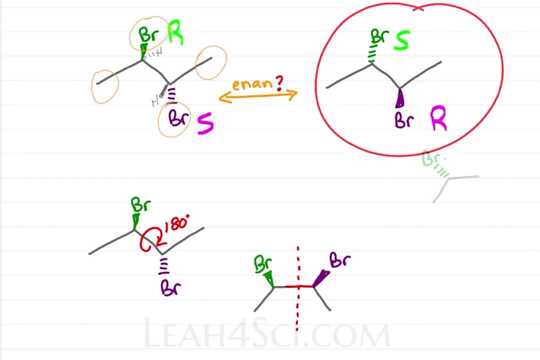 each other. out thing for this molecule, where I keep the left the same, and for the right. methyl goes down in the plane of the page. bromine wedge down is now dash up and, once again, internal symmetry. If we bring them side by side they appear to be mirror images of each other. 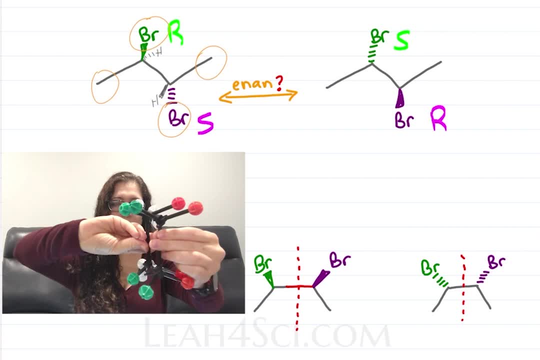 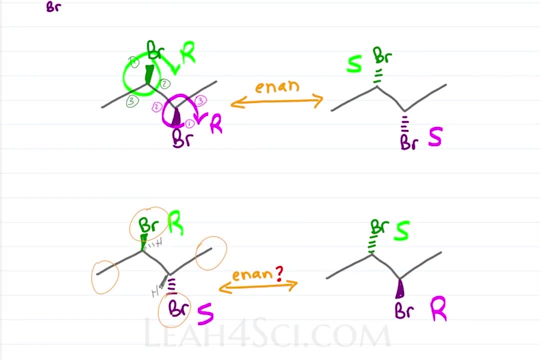 but if I flip this molecule, as I did with a model kit, they are perfectly superimposable on each other and that makes them the same exact thing. Going back to our original example, no, these are not enantiomers. it's exactly the same thing. and if they're exactly the 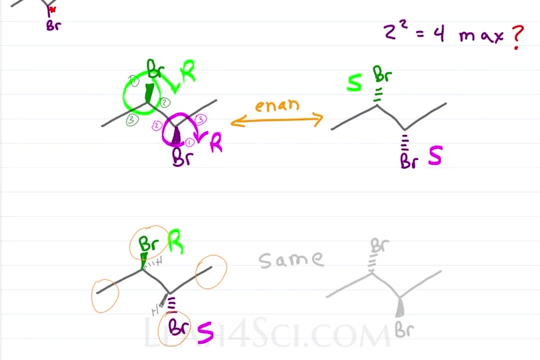 same, we have a total of 3 rather than 4 stereoisomers. So what about this equation? 2 to the n equals 4 max, but the mesocompound costs us 1.. How do you recognize mesocompound 1, the chiral? 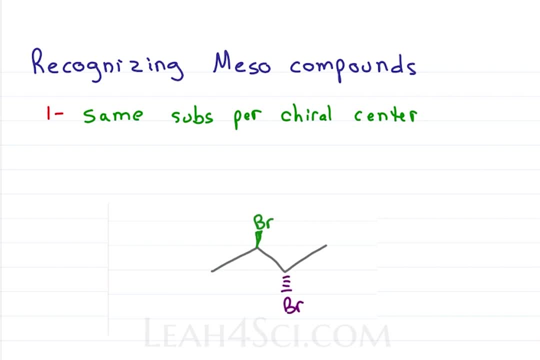 molecule has the same exact substituents on each chiral center and 2, they have the opposite chirality: 1 is R, the other is N, 1 is S or one is S and the other is R. But this is the long way, The faster way which. 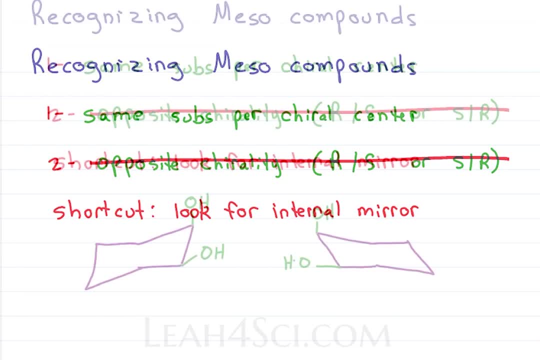 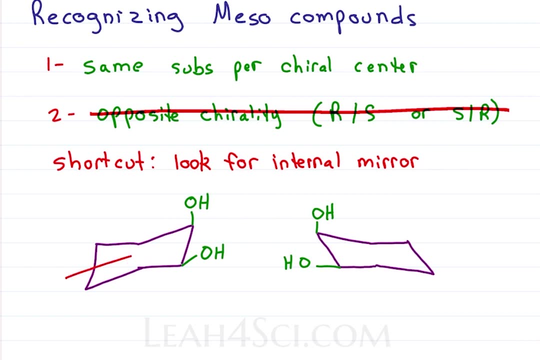 isn't always possible is to look for that internal mirror. Take these chair conformations, for example. The molecule has two OH groups, but we can't necessarily see an internal plane of symmetry. What I can tell is that the two molecules are mirror images of each. 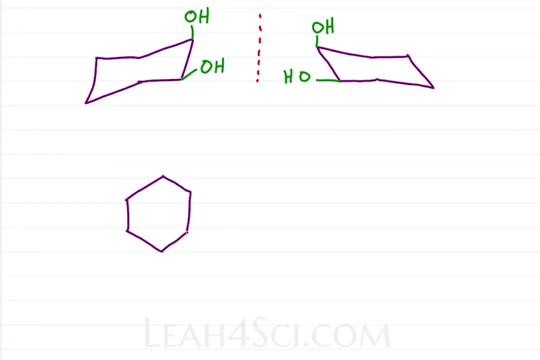 other, and so they are potential enantiomers. When in doubt, flatten it out. If you didn't immediately recognize that the OHs going up means that they're internally symmetrical, just flatten it out. We'll make these carbons 1 and 2, and put both OHs on a wedge, since 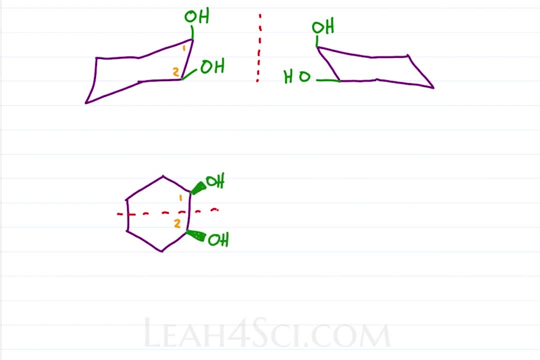 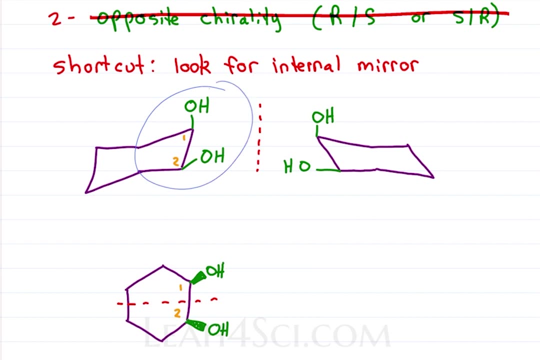 they're coming up and out of the chair and look at that Internal plane of symmetry, mesocompound. Or you can go back to option 2 and find R and S on your chair conformation or on your flattened structure. R and S with identical substituents once again confirms.